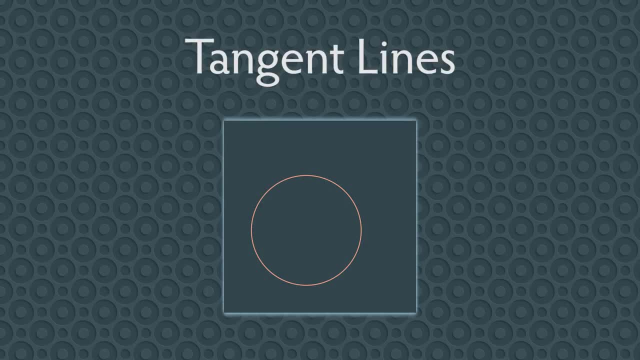 Tangent lines have been studied for more than 2,000 years. Originally, a tangent line was defined to be a line that touched a circle at just one point, But over the centuries this definition has been expanded to include lines touching other curves and not just circles. 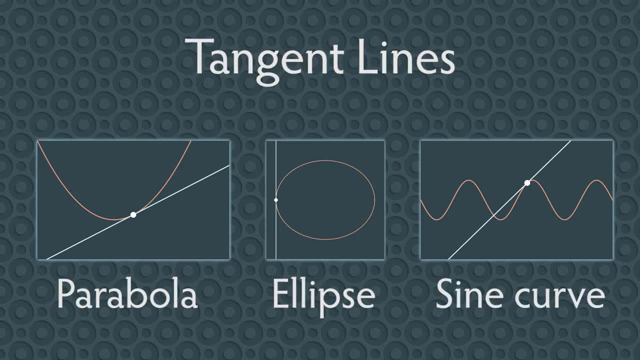 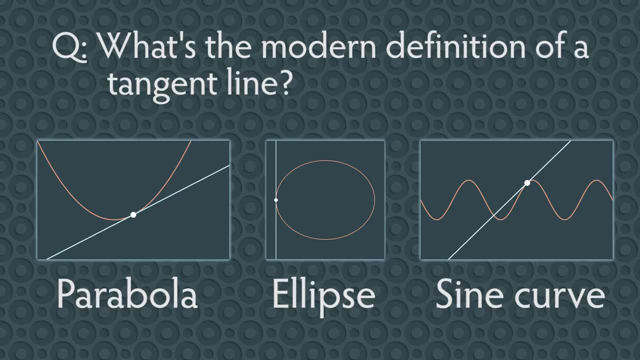 You can have a tangent line to a parabola, an ellipse or more elaborate curves like the sine curve. So what's the modern definition of a tangent line? Well, math definitions are tricky things. They're kind of like wishes you make to a genie If you're not. 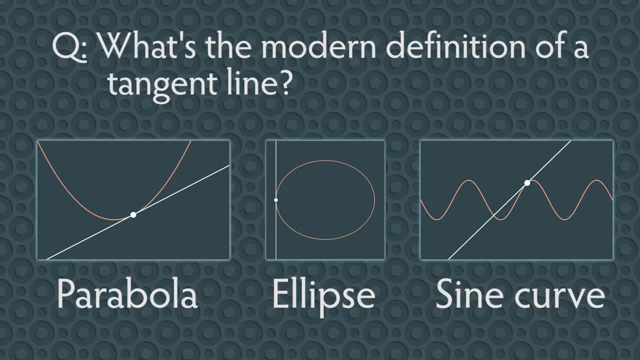 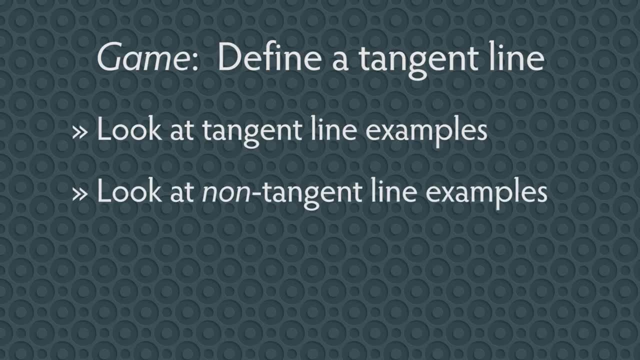 very careful with your choice of words. you can end up in trouble. So let's play a game. I'm going to show you a bunch of images of tangent lines and non-tangent lines. While I do this, try to come up with your own definition of a tangent. 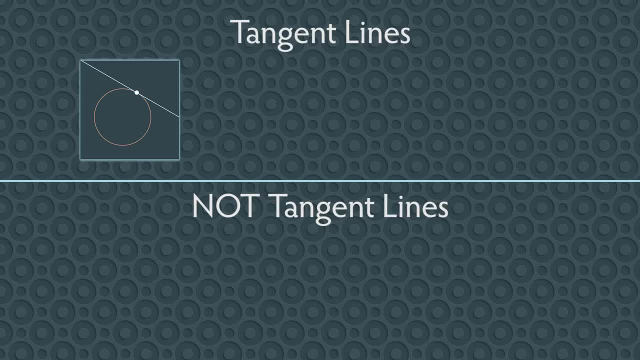 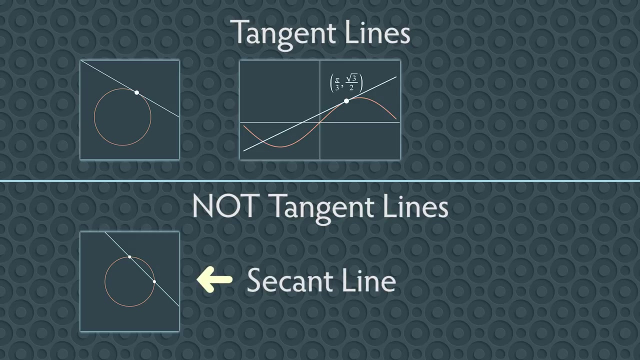 line. Here we have a line that touches a circle at only one point. This is a tangent line. And here we have a line that crosses a circle at two points. This is not a tangent line, We call this a secant line. And here is a line that touches the sine curve at the point. 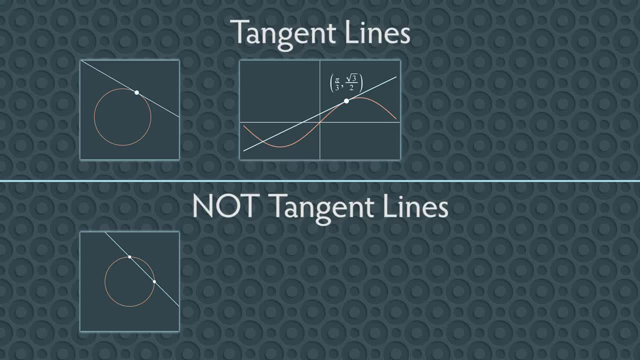 pi over three, the square root of three over two. This is a tangent line. This line also goes through the point pi over three, the square root of three over two, But it's not a tangent line. Here's a tangent line that touches a cubic curve at only one point. Notice. 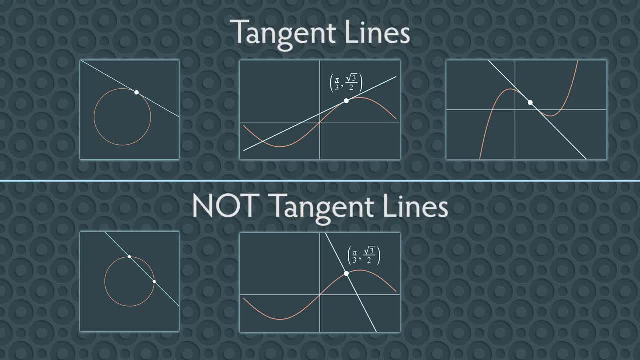 how part of the curve lies above the tangent line and part of the curve lies below it, And here we have a line that touches the graph of y equals the absolute value of x only at the origin, but this is not a tangent line. 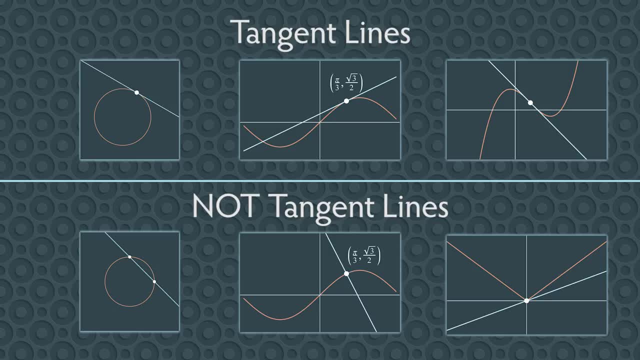 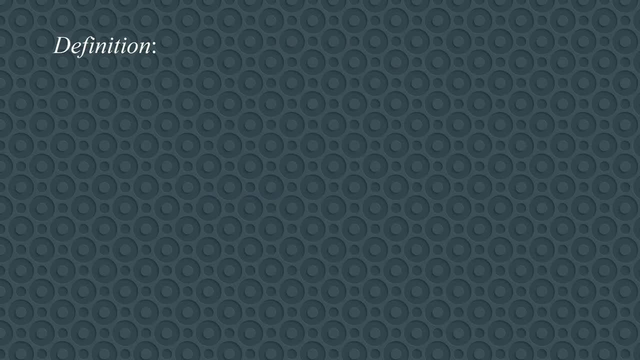 So here we have six examples, three tangent lines and three non-tangent lines. From these six examples, how would you define a tangent line? A common definition, you might hear, is a tangent line to a curve is a line that touches the curve at only one point. 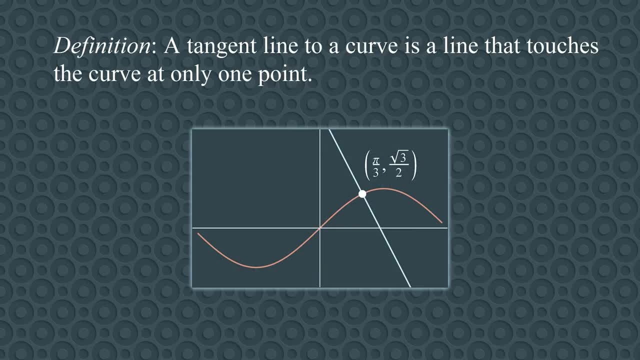 But this definition is wrong. This line touches the graph of the sine curve at only one point, but it isn't a tangent line. The problem here is that the line crosses the curve rather than gradually approaching it before touching it at one point. 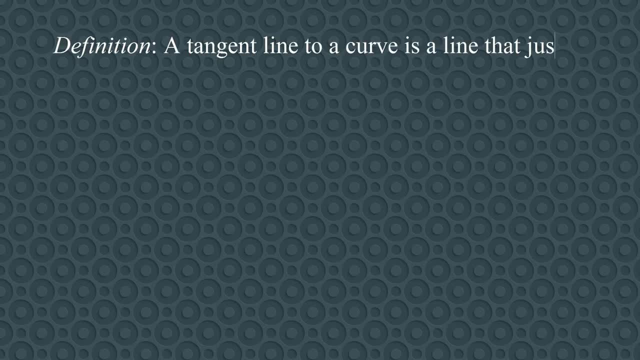 Let's try again. A tangent line to a curve is a line that just touches the curve at only one point. This definition is better. It captures the idea that a tangent line gradually approaches the curve and touches it at a single point. but it's also wrong. 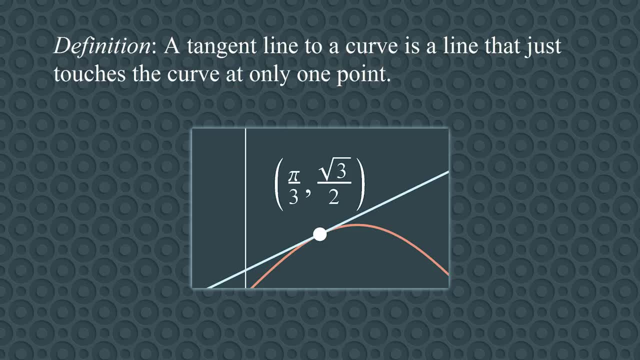 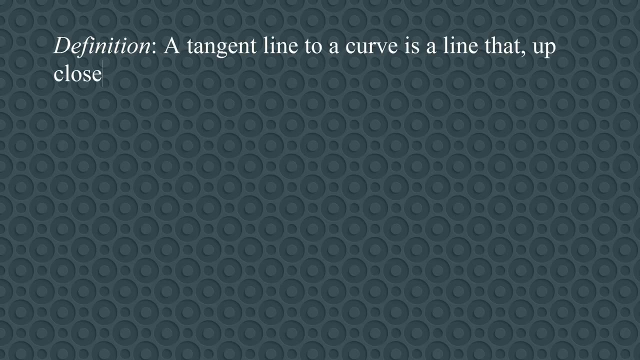 Look again at the sine curve example. Up close the line does just touch the curve at one point without crossing it. but if you zoom out you will see the line crosses the curve a second point farther away. So a better definition might be: a tangent line to a curve is a line that, up close, just 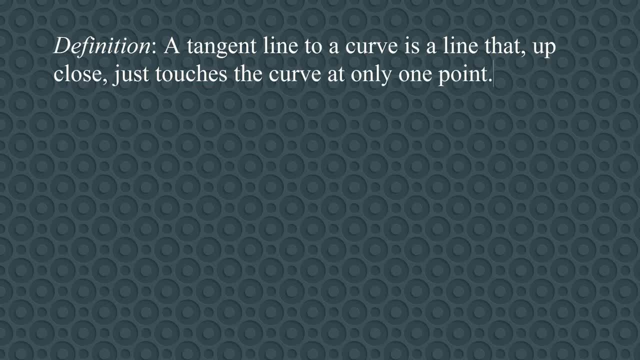 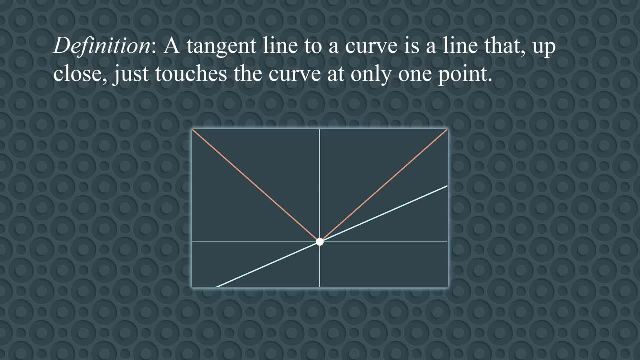 touches the curve at only one point. This is a pretty solid definition, but the phrases just touches and up close are both kind of vague. For example, look at the graph, for y equals the absolute value of x. There are lots of lines that only touch the graph at the origin, but none of them are. 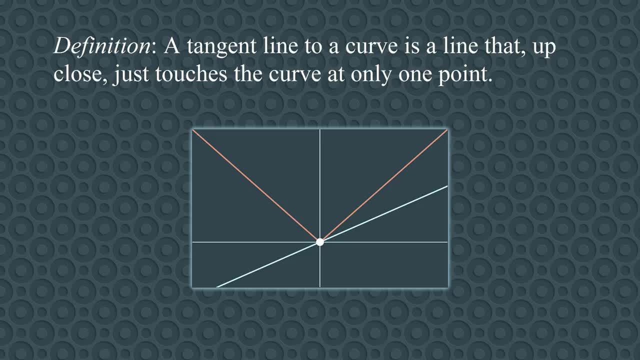 tangent lines. What is it about these lines that prevent them from just touching the curve? One thing to notice is that you can rotate the line back and forth and it still only touches the curve at the one point, But in the example of the tangent line to the sine curve, this does not happen. 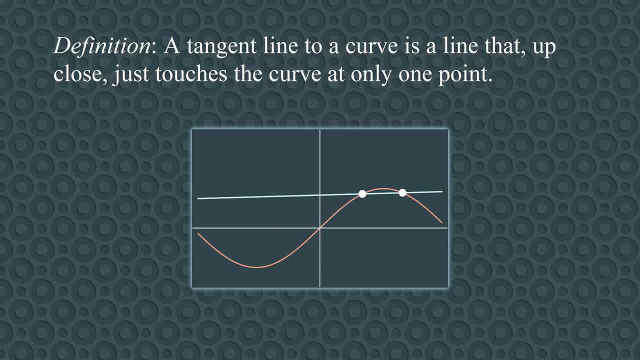 If you rotate this tangent line even slightly, it will become a secant line and cross the curve at another nearby point. Remember, a secant line is a line that passes through two points on a curve. With this in mind, we can try to make the definition more precise. 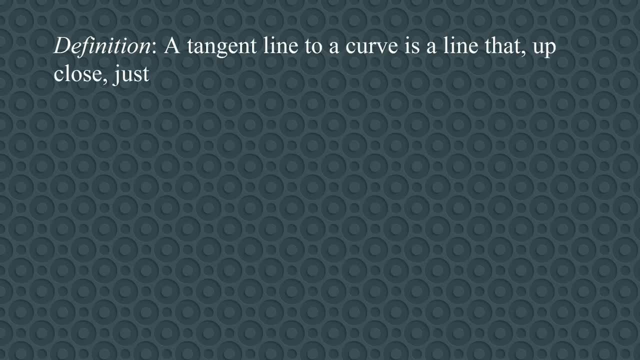 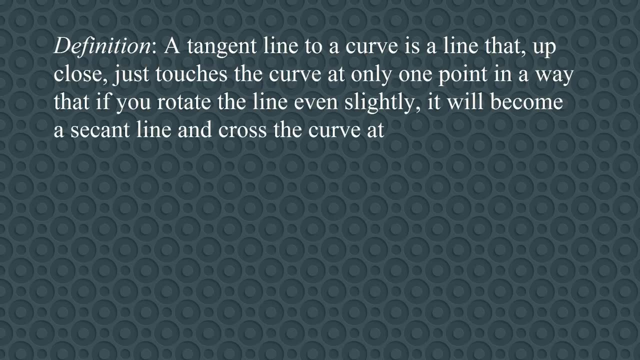 A tangent line to a curve is a line that, up close, just touches the curve at only one point, in a way that if you rotate the line, even slightly, it will become a secant line and cross the curve at a second nearby point. 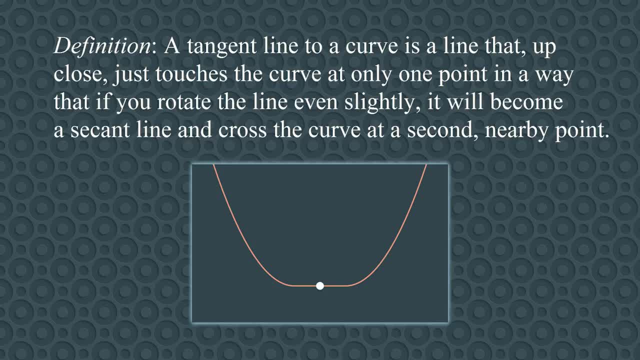 But even this definition runs into problems if the curve flattens out on either side of the point. At this point things are getting a bit ridiculous. but that's mathematical. It can take years and years of hard work just to find the right definition. 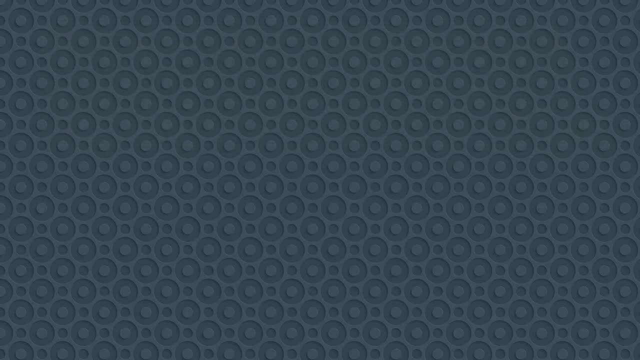 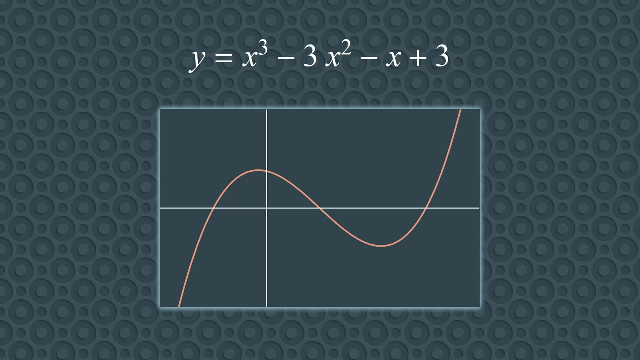 Using calculus, however, we can give a much simpler definition for a tangent line. As an example, let's use the graph of: y equals x cubed minus 3x squared minus x plus 3.. We'll use the idea of limits to define the tangent line to the point. 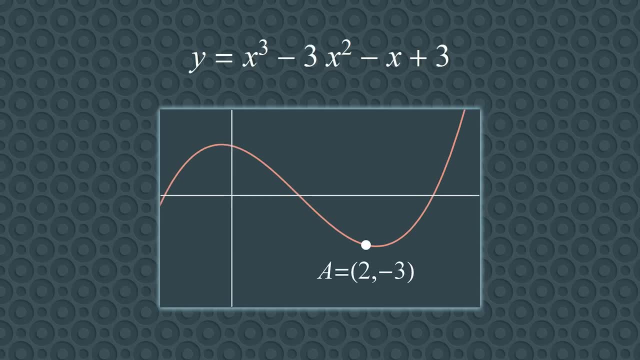 We'll call this point A. First, let's get a closer look. Here's the idea. Pick a nearby point, Let's call it P. You can pick P to be to the left or to the right of the point A, It doesn't. 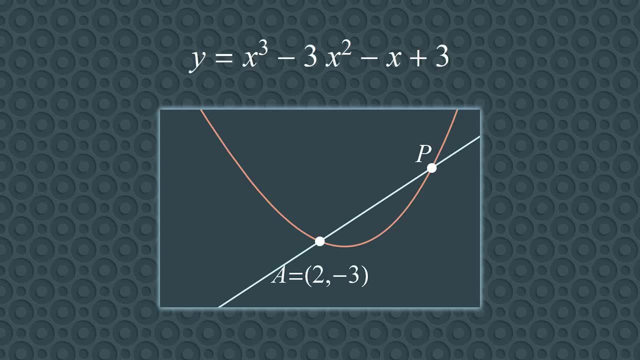 matter Now. if you draw a line through P and A, you get a secant line. If you let P get closer and closer to the point, the secant line gets closer and closer to the tangent line. Once P hits, the secant line becomes a tangent line. 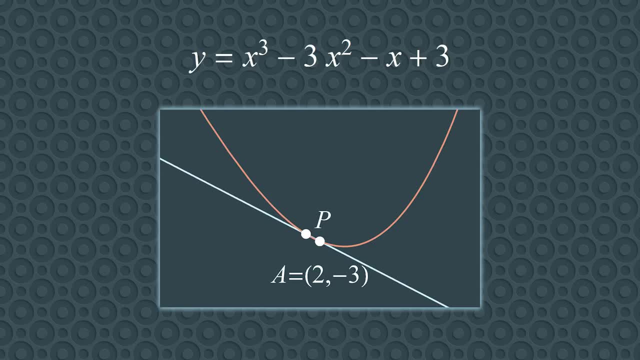 And if you let P approach our point from the other direction, you get the same answer. It's OK to set both of the pointersare. You can then draw a line to the point where we've got the third and fourthtır。」. 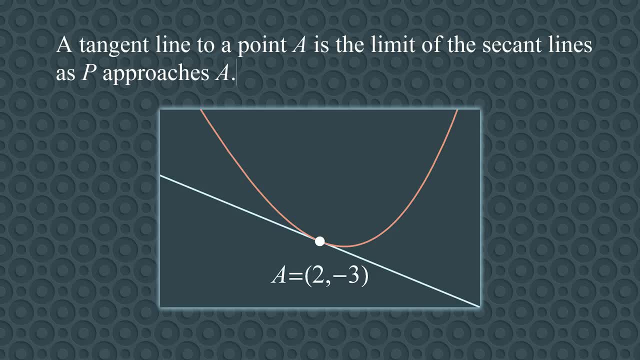 So you can define the tangent line to A as the limit of the secant lines as P approaches. This is the calculus definition of a tangent line. A tangent line to point A is the limit of the secant lines as P approaches A. The two key things are these: 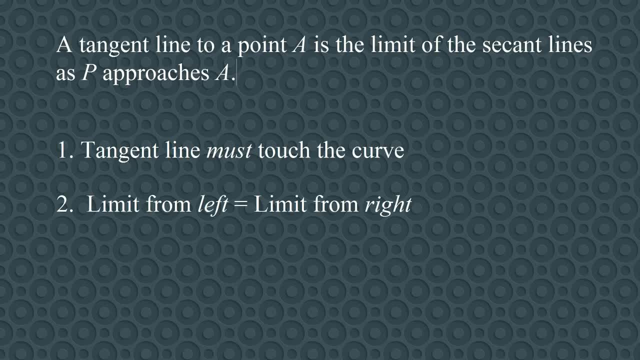 First, the tangent line must touch the curve at the point And second, the limit of the secant lines should be the same regardless if you approach from the left or towards. ranged from right to left, should be equal to a half of a half of the mass. 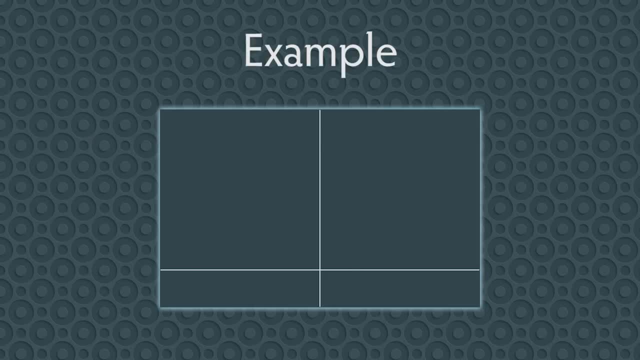 Both a half of a second line, except for the secant line or the right. Let's see some examples to show you why you need to be careful with this definition. First look at the graph of f of x equals sine x over x. 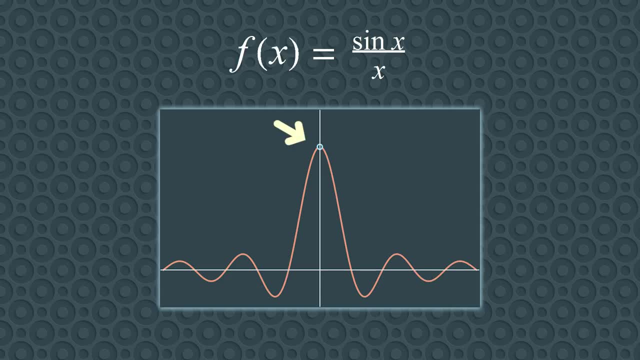 What is the tangent line to the point? You could use the method of picking a nearby point P and letting it approach the point, And if you approach from the right you get the same answer In both cases. the limit of the secant lines is the horizontal line. y equals 1.. 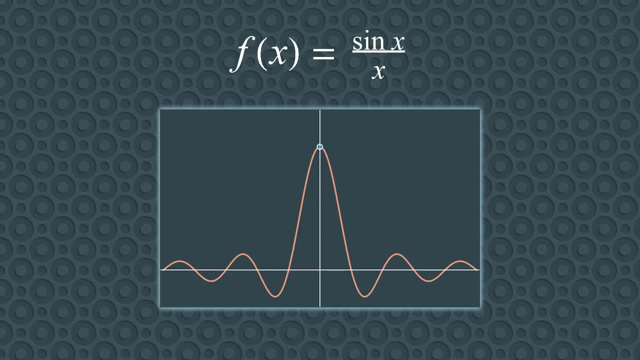 This line, however, does not touch the curve. This is because the point is not on the graph, since if you plug in x equals 0 into f of x, you get division by 0. So this curve does not have a tangent line at the point. 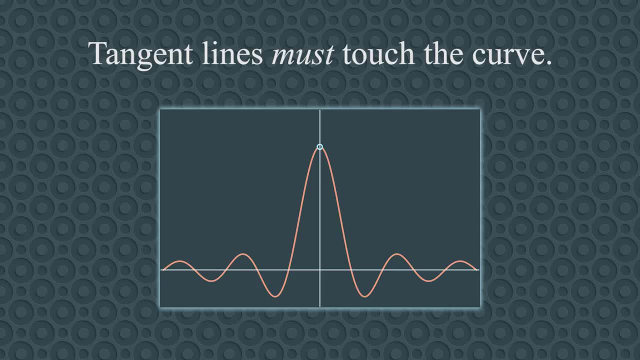 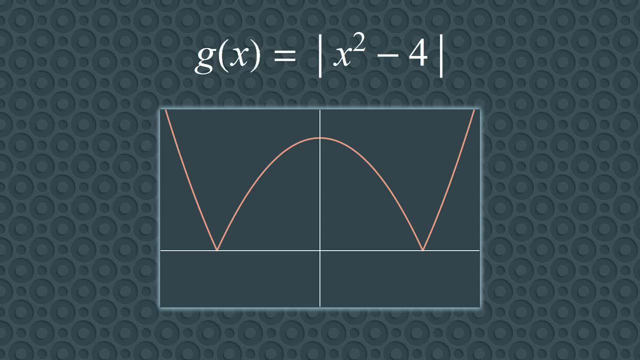 This example highlights the fact that tangent lines must touch the curve. Next look at the graph of the function When g of x equals the absolute value of x squared minus 4.. Let's find the tangent line to the point. If you let P approach the point from the left, the secant lines approach the line. 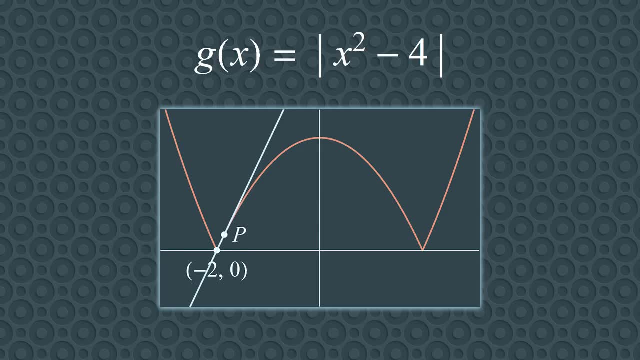 But if you let P approach the point from the right, the secant lines approach a different line. So you get different lines depending on your direction of approach. The limit from the left is different than the limit from the right Because the left-hand and right-hand limits are different. we say the limit does not exist. 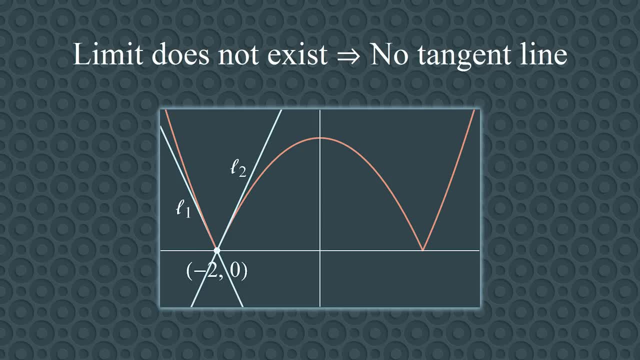 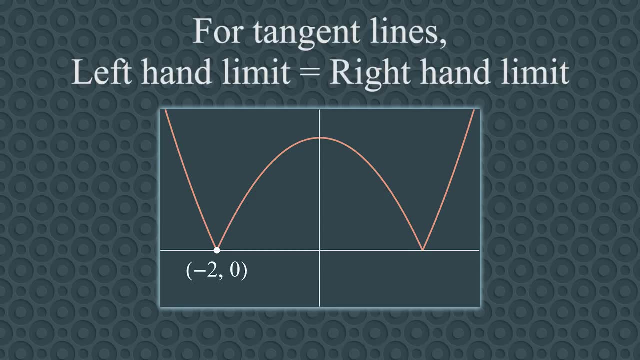 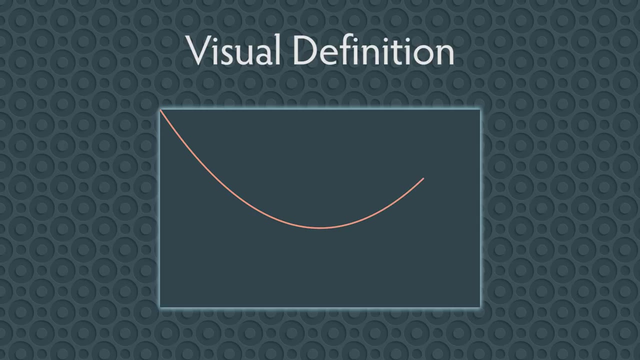 So there is no tangent line to the point. This example shows the importance that the limit of the secant lines should not depend on the direction of your approach. The left-hand limit and right-hand limits should be the same. I'd now like to give you a different, more visual way to think about tangent lines. 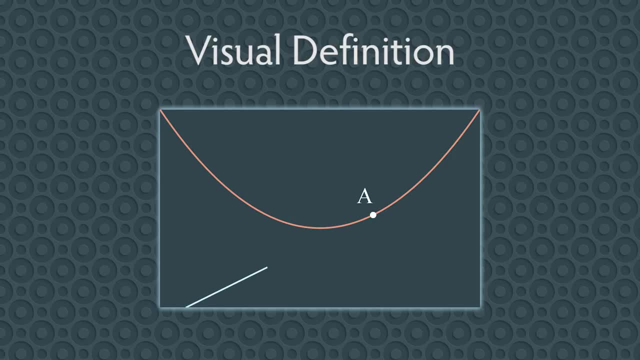 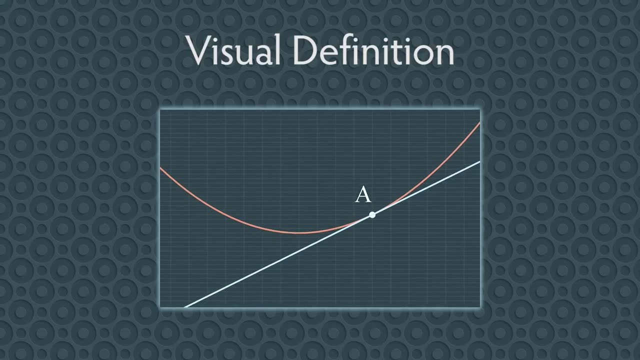 Here's the graph of a parabola. Let's go ahead and draw the tangent line to the point. Watch what happens if we slowly zoom in on this point. The closer we get, the more indistinguishable the curve and the tangent line become from. 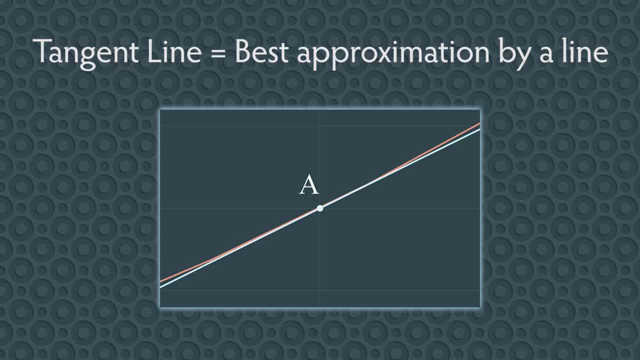 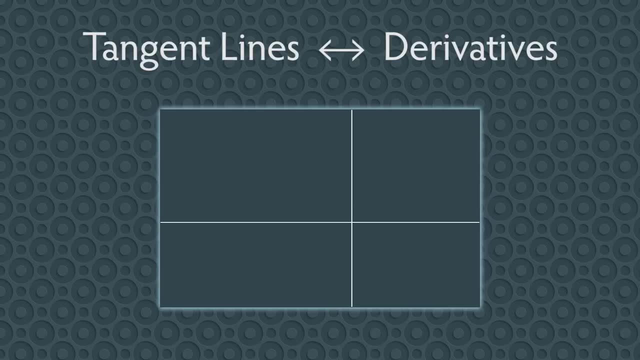 one another. This is another defining feature of the tangent line. It's the line that is most similar to the curve at the point. Now that we know what tangent lines are, let's talk about the connection between tangent lines and derivatives On this curve. the tangent line at is the limit of the secant lines as P approaches. 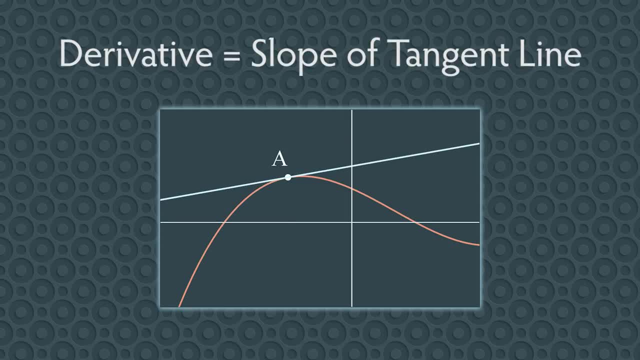 A. The derivative is simply the slope of the tangent line. It's a number, not a line. Think of it as measuring the steepness of the curve. at the point A, Like the tangent line, you compute the derivative using limits. You begin by finding the slope of the secant line through A and P: The slope M of a line. 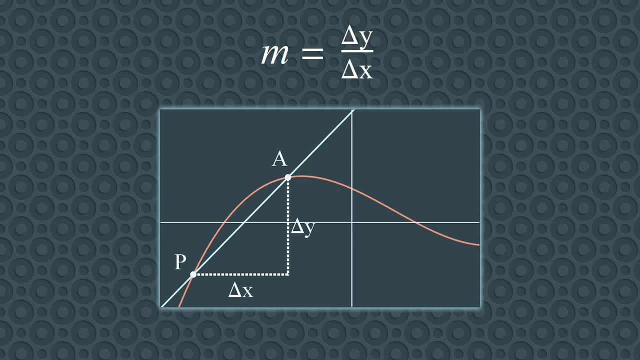 is the change in Y over the change in X. We use the capital Greek letter, delta, to stand for difference a. the secant lines approach the tangent line and the slopes approach the derivative. There are several ways to write the derivative, but a common way is dy over dx. 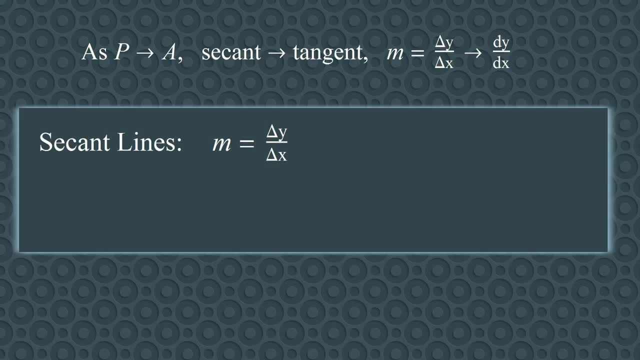 Be careful that you use deltas for the slope of a secant line and ds for the slope of the tangent line. Delta x and delta y are actual numbers, whereas dx and dy are called differentials. They're not really numbers, but you can usually think of them as infinitely small numbers. 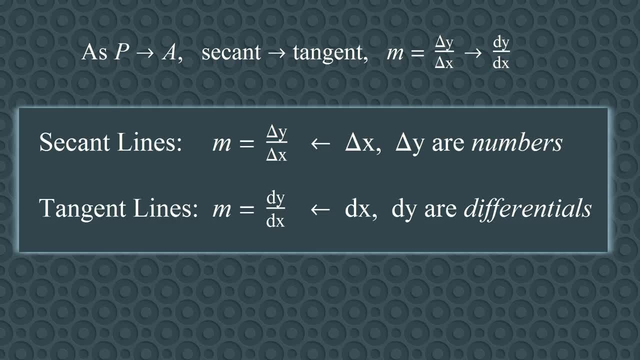 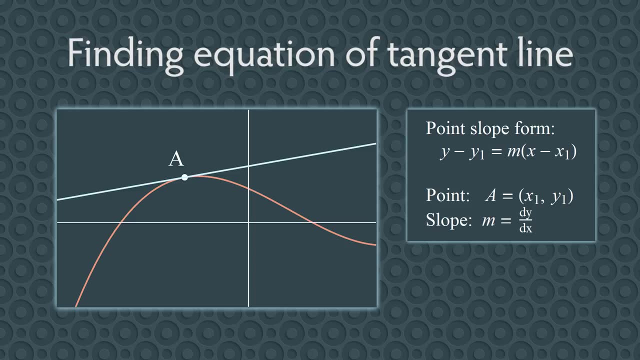 sometimes called infinitesimals. This notation will come in handy a lot in calculus. Once you know the derivative, you can find the equation of the tangent line. This is because to find the equation of a line, you either need two points on the line. 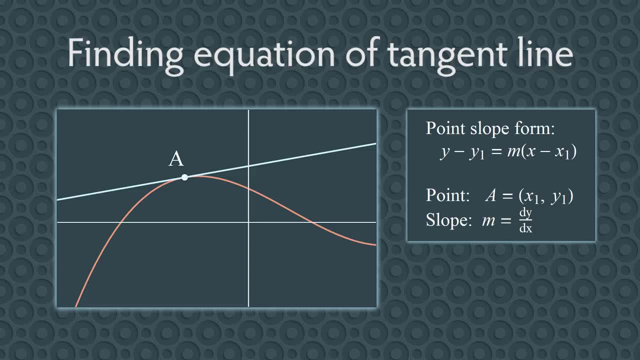 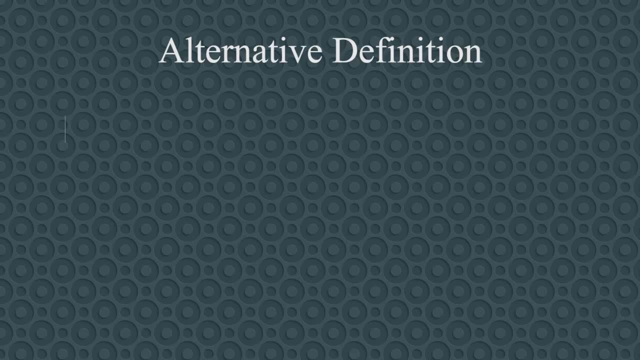 or one point and its slope. In this case, we have one point a and the slope dy over dx. In fact, this is another way to define the tangent line. The tangent line through a point a is the line that passes. 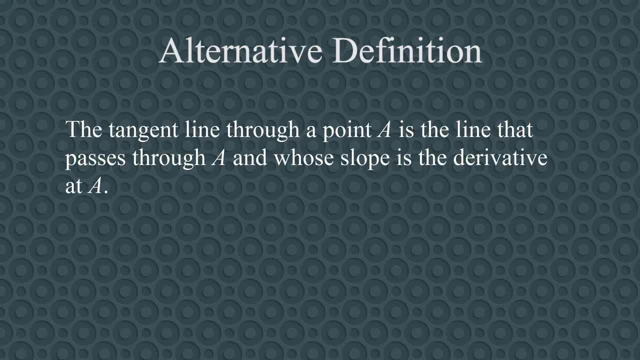 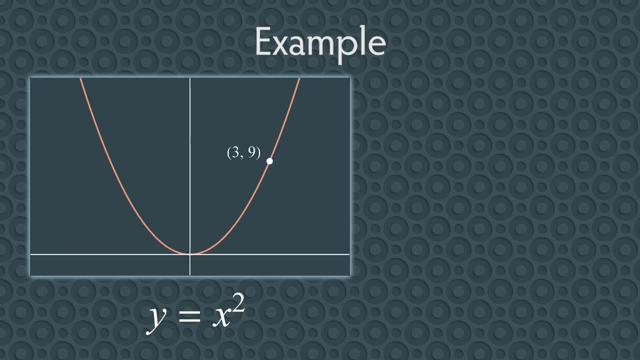 through a and whose slope is the derivative at a. This means the same thing as our earlier definition. It just hides the process of taking a limit by saying the slope is the derivative. Let's now see an example. Suppose we want to find the equation of the tangent line to the parabola. y equals x squared. 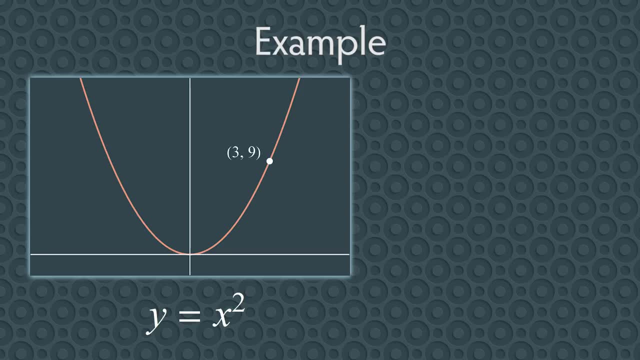 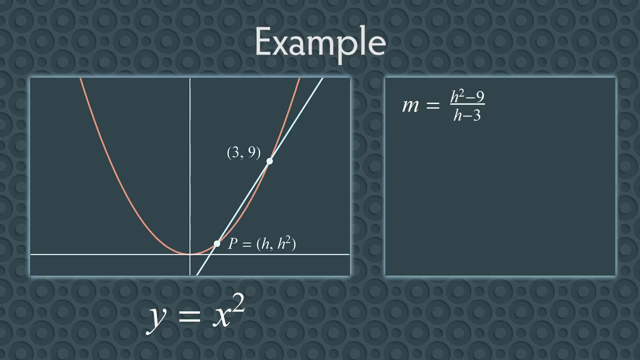 at the point. We do this by picking a nearby point, P. We'll call the x-coordinate h, which means the y-coordinate is h squared. The slope of the line is the slope of the tangent line, The slope of the line through and is h squared minus 9 over h minus 3.. 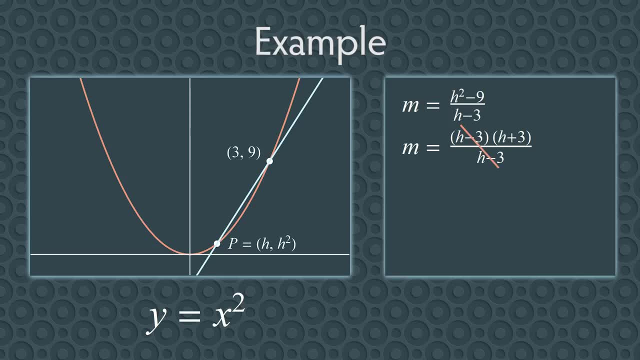 We can simplify this expression by factoring the numerator, then canceling. So the slope of this secant line is h plus 3.. Next look at the limit as P approaches the point. We do this by letting h approach 3.. 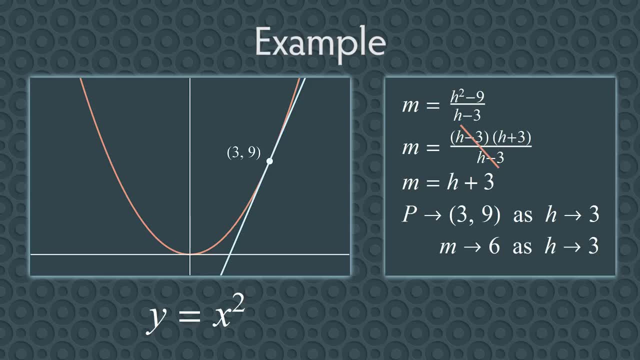 As h gets closer to 3,, the slope approaches 6.. So we now have a point. The point is 3, 9, and the slope is 6.. The point-slope form for a line is: y minus y1 equals m times x minus x1, where x1, y1. 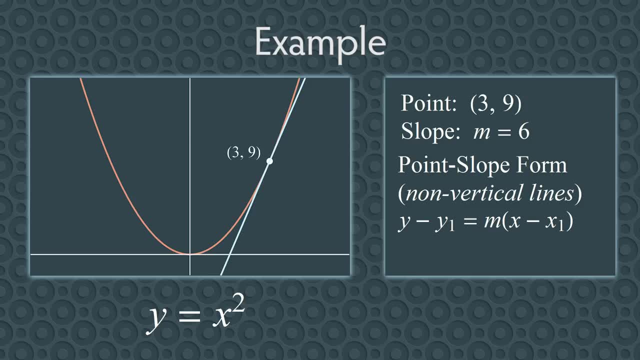 is any point on the line. This only works for non-vertical lines. Vertical lines all have the form x equals x1.. Now plugging in our values gives us y minus 9 equals 6 times x minus 3.. We can leave it like this or rewrite it in the more common form by solving for y: 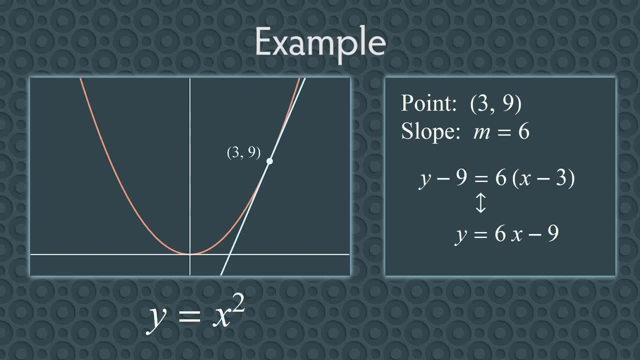 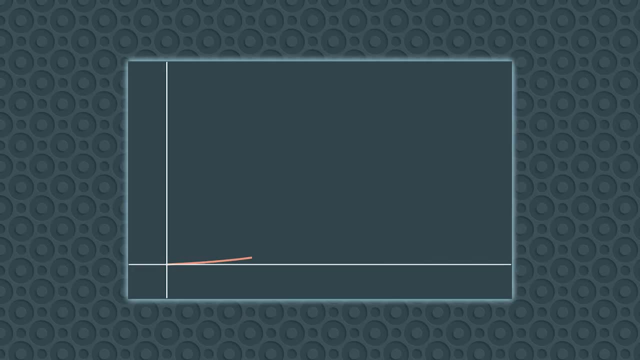 If we do that, we get y equals 6x minus 9.. This is the equation of the tangent line to the point. If you don't mind, I'd like to go off on a tangent for a moment and touch on an important.